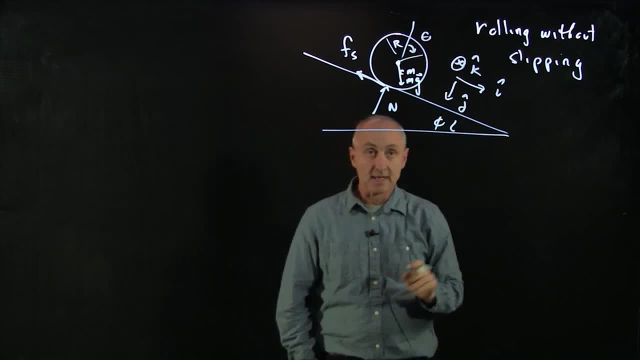 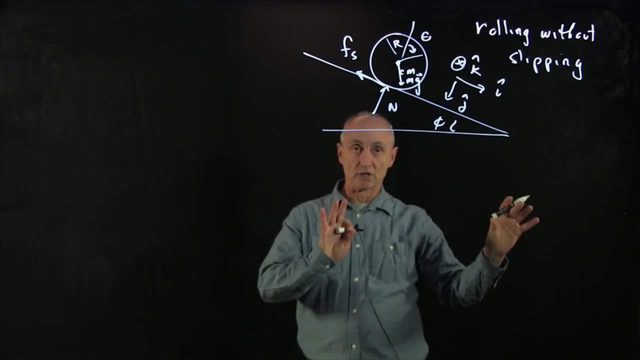 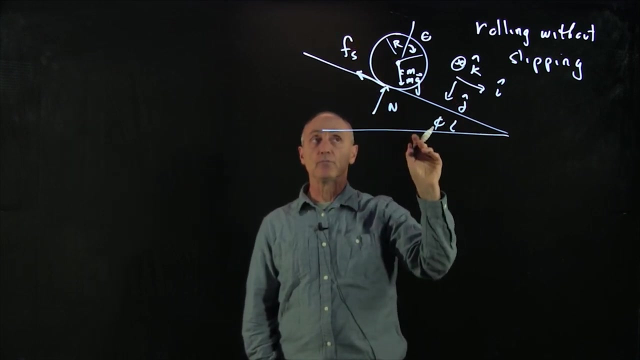 and that will correspond to some angle theta. Now here we're now going to enlarge how we apply both translation and rotation, And the beauty of this problem is we now can decode our motion into translational motion and rotational motion. So for the translational, 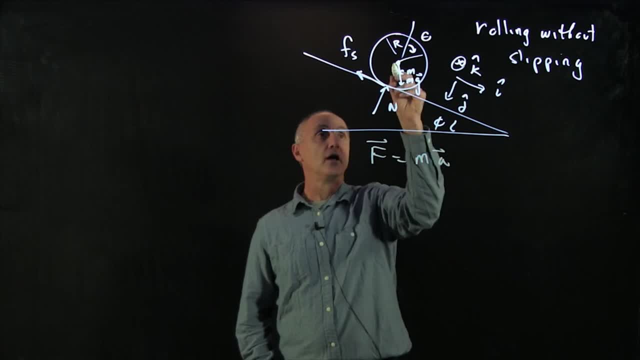 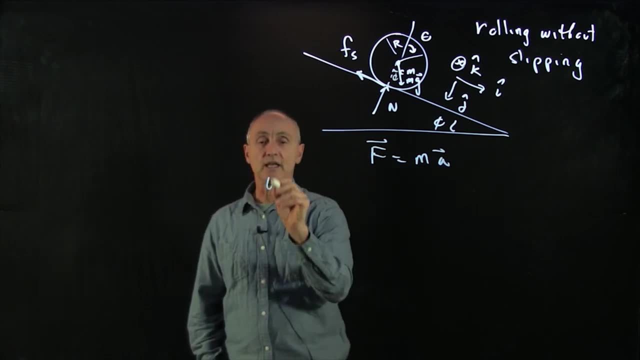 motion, we'll apply Newton's second law. Now, if this is the angle phi, then that's the angle phi as well, And so our forces in the i hat direction. we have mg sine phi minus the friction force, and that's equal to the x component of the acceleration. 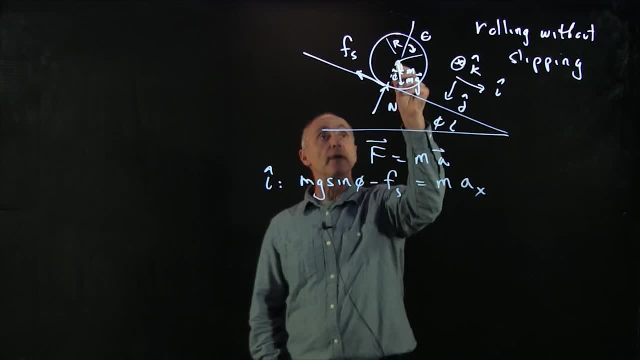 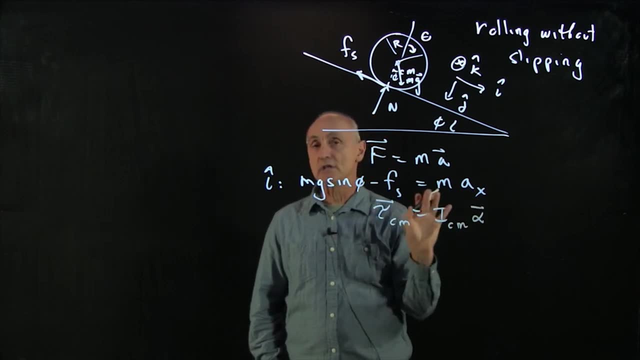 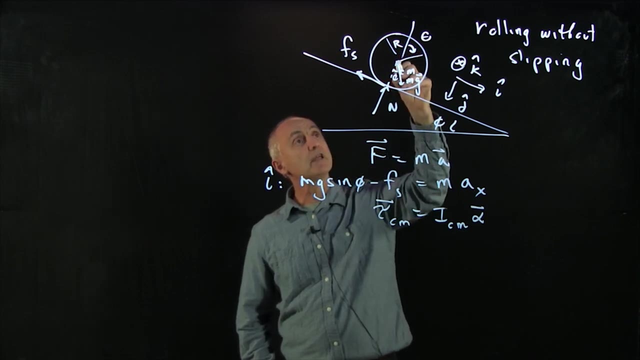 Now we also can choose the center of mass to calculate the torque, And so what we're really just studying here is simply our old problem in the center of mass frame of fixed axis rotation, And you can see, gravity is acting at the center of mass, so it produces. 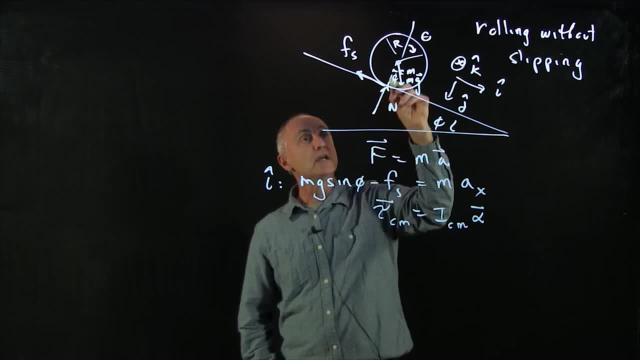 no torque about the center of mass. The normal force is directed towards the center of mass. and so when we take that vector product of the vector product, of the vector product of r, cross n from cm to this point down, here the contact point, these forces are antiparallel. 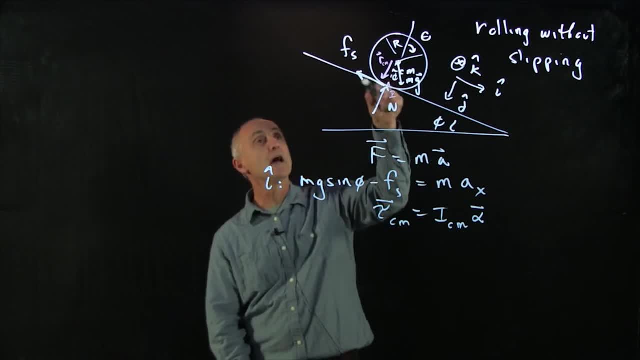 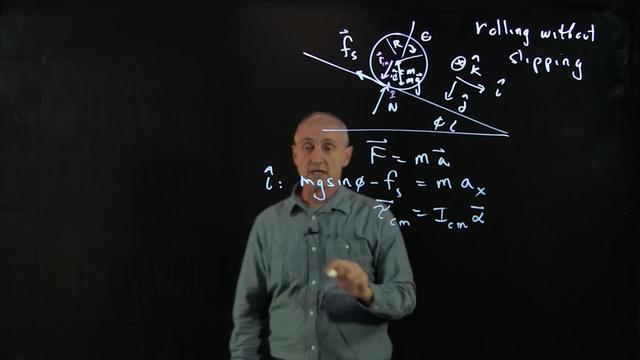 so the normal force produces no torque And the only torque that we have is from the friction force, and that friction torque is going to give us a positive angular acceleration in the k hat direction. It's at right angles with the vector r, so we have fs times r equals. 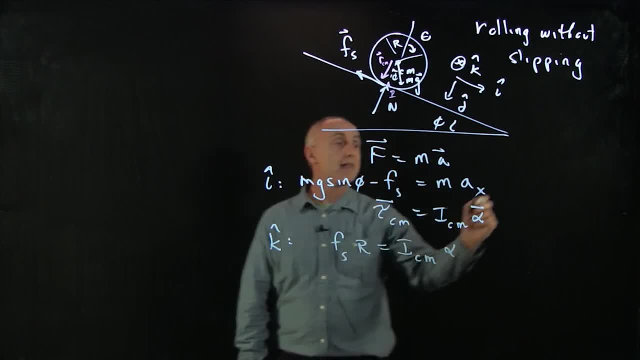 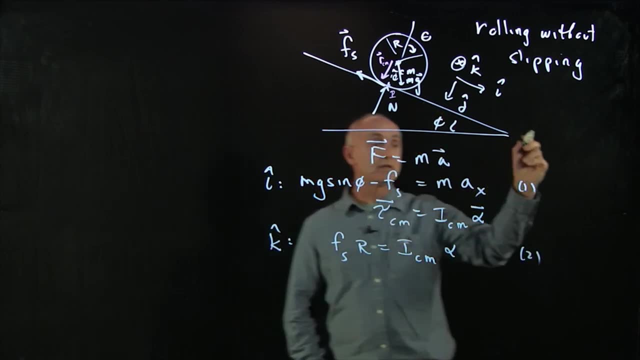 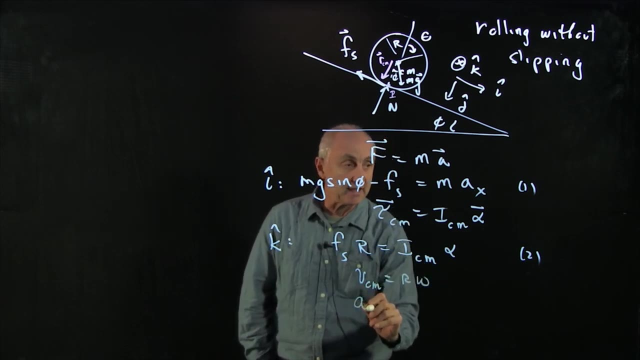 i, center of mass times, alpha, And these are our two dynamic equations. But remember, when the object is rolling without slipping, let's just remind ourselves that vcm equals r omega and if I differentiate, the acm, which is what we're calling ax, is equal to r alpha. 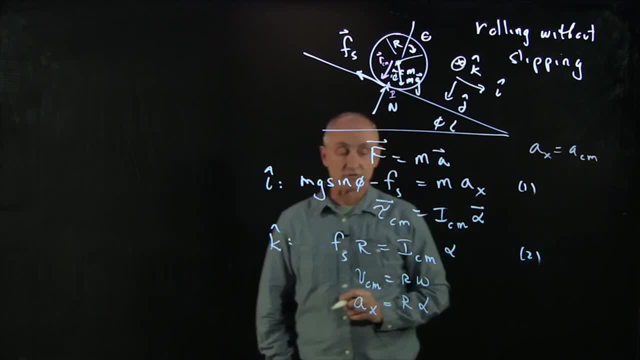 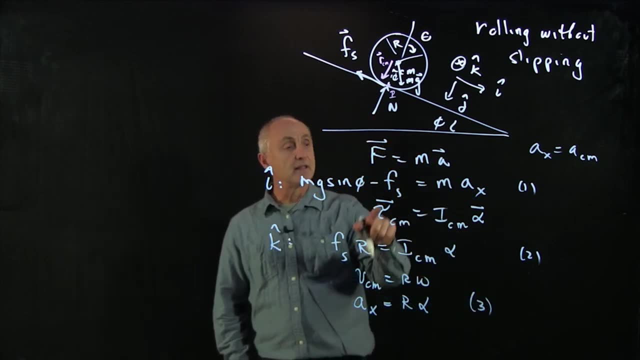 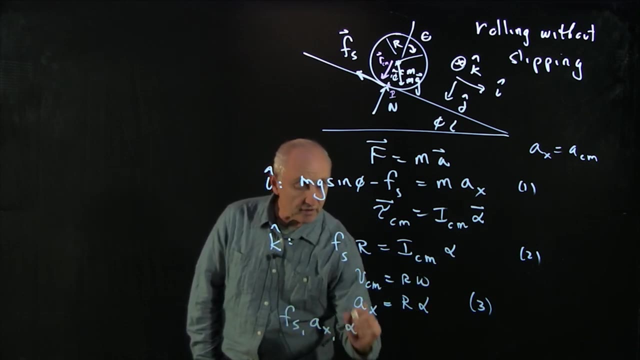 So this ax here is the acceleration of the center of mass, And that's our center of mass. And then we have the third condition. And so now I see that I have three equations in my unknowns: fs, ax and alpha, and so I'm going to solve these equations for a. 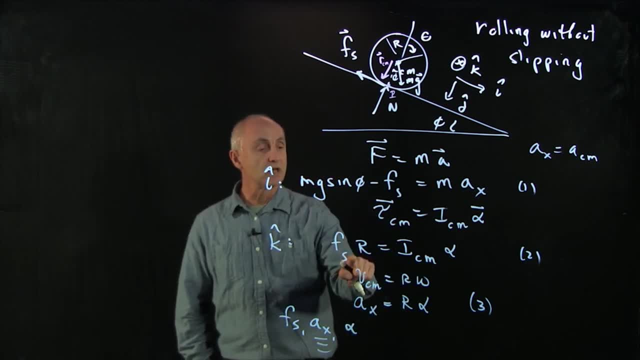 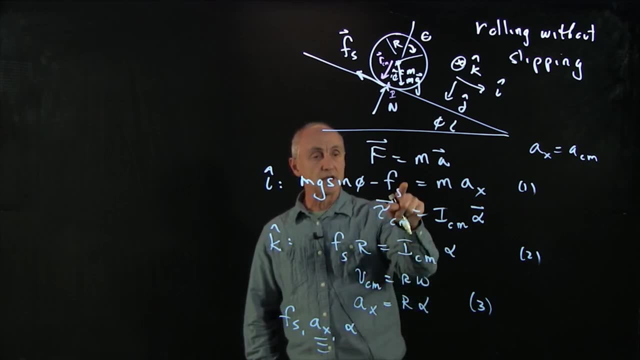 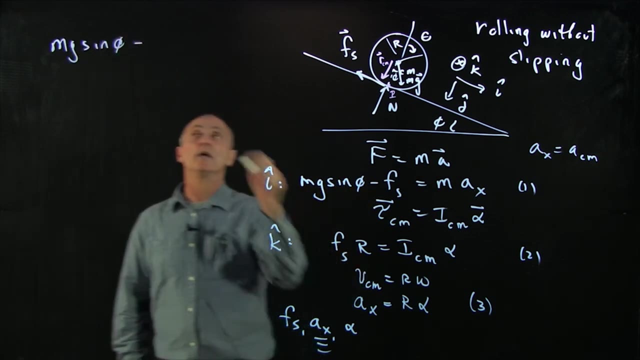 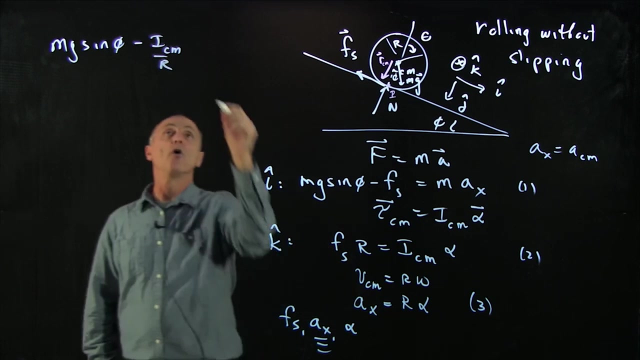 And I'll look at these equations and what I'll do is I'll just substitute for alpha ax over r and then solve this equation for fs and put it in there, And so I get mg sine phi. Now my fs is equal to icm over r times alpha, But alpha is ax over r, So 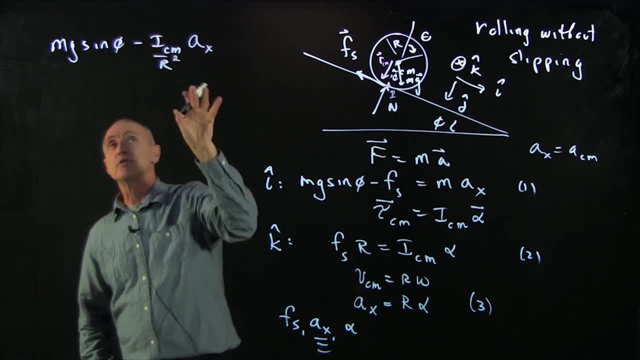 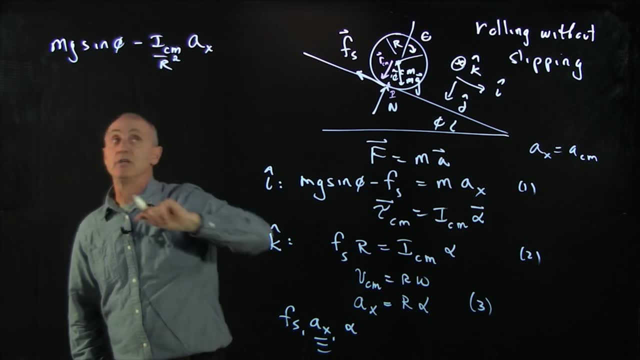 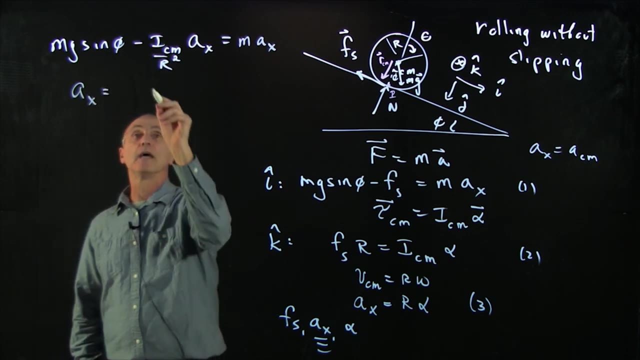 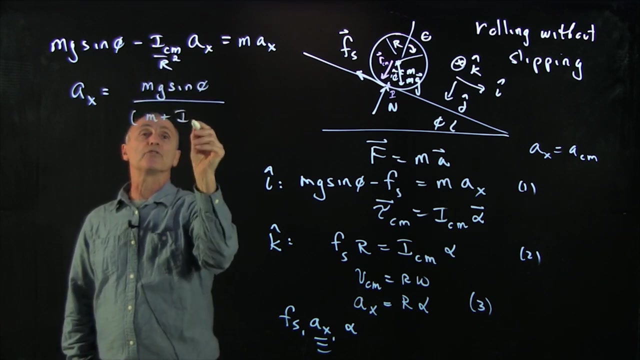 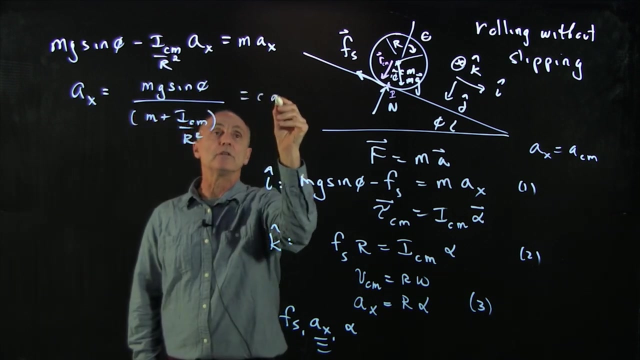 that's ax and an r squared. Notice, dimensionally i is mr squared. So this is just ma, the dimensions of force, mg, dimensions of force, And that's equal to max. And now I can solve for ax over r and I get mg sine phi divided by m plus icm over r squared. Now ax is a constant. 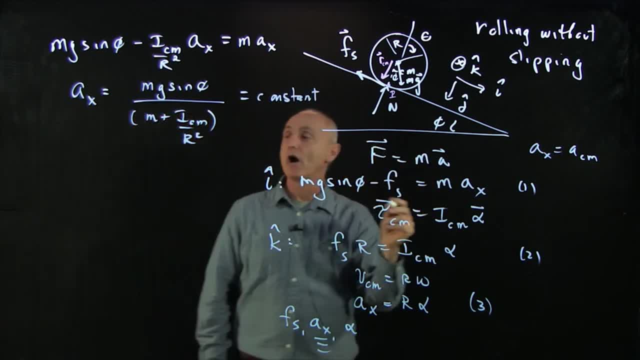 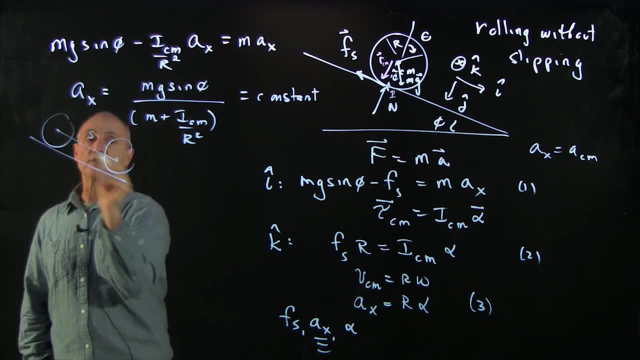 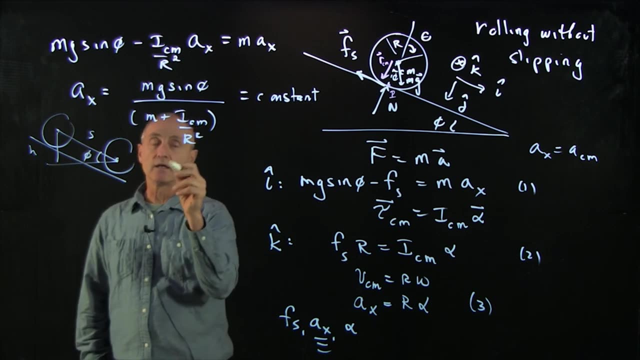 And from our kinematic equations, if our object is moving a distance s as it drops a height h, We know from kinematics and we could work this out, we have that the x cm is one half a cm t squared, and we know that that the velocity v cm equals. 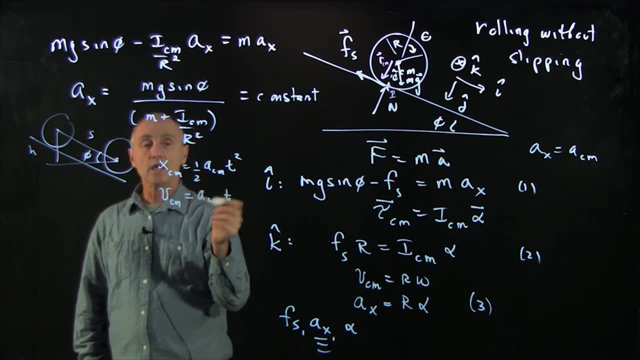 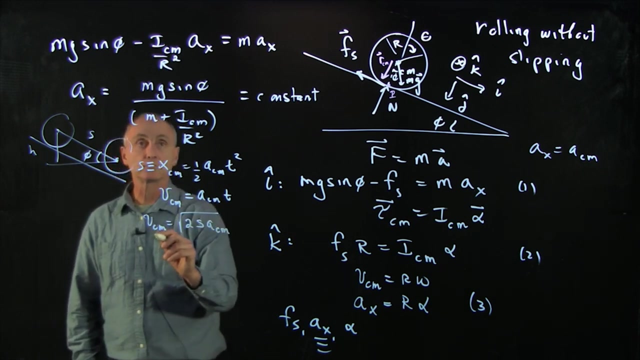 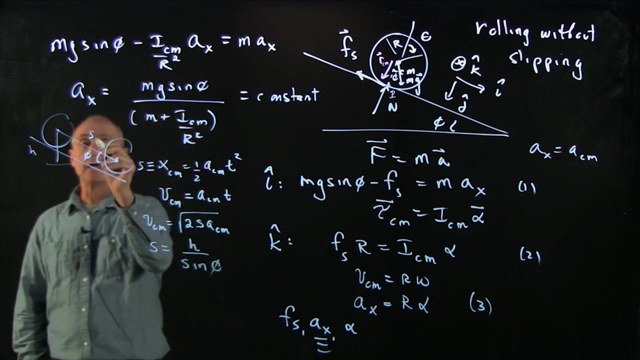 a cm times t, And so when we put these two together, this is the distance s, we get that the velocity cm is equal to the square root of 2 s times a cm. Now s is equal to h over sin phi, h over s is sin phi, And so v cm. 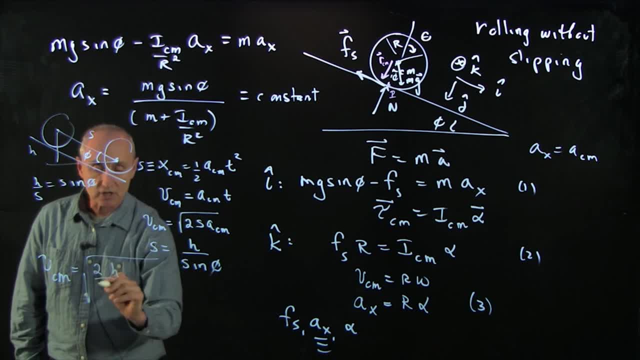 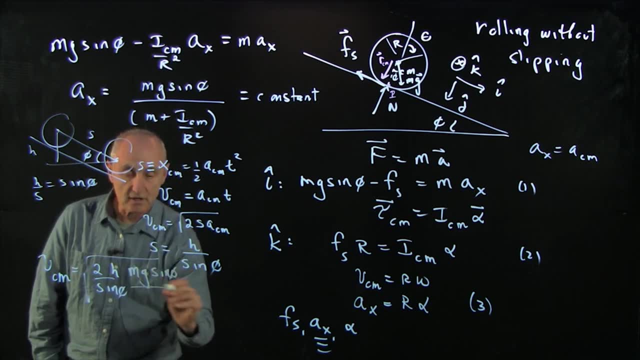 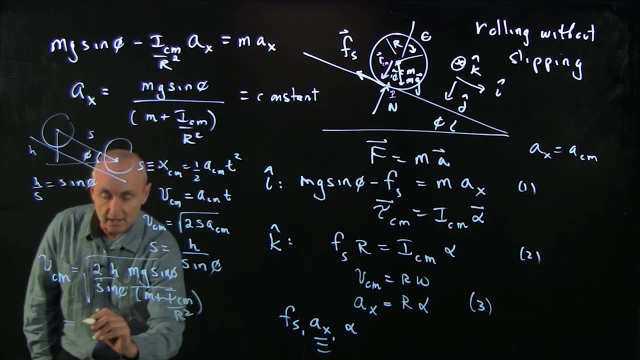 equals a cm, the square root of 2h sine phi times ACM. but we've solved for ACM mg sine phi over m plus ICM over r squared, and so we get the square root of 2mgh over m plus ICM divided. 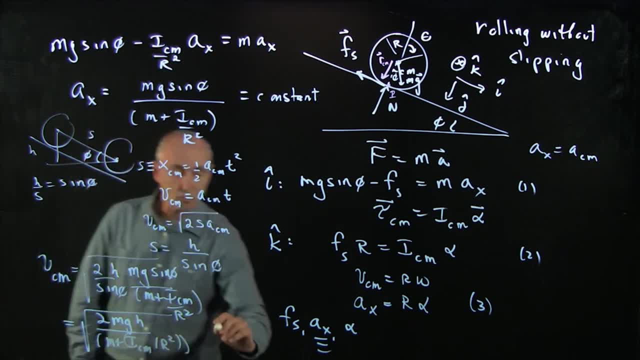 by r squared, and this agrees with our energy method.